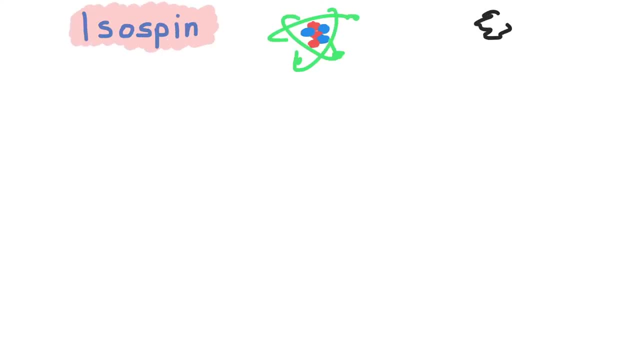 Isospin is a concept that appears in particle physics. We use isospin to distinguish between two possible states of a system. The origin of the word isospin comes from the greek isos, which means equivalent, and spin, which plays an important role in quantum mechanics. 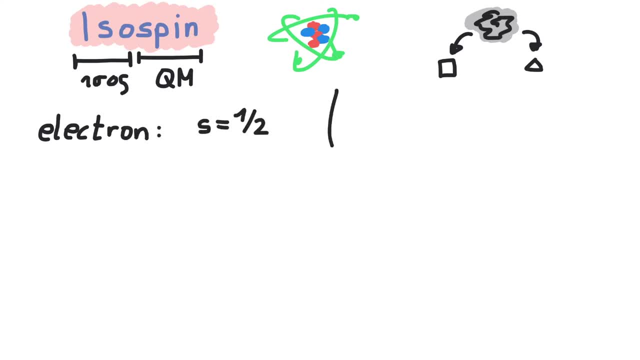 For example, an electron is a spin one-half particle. Its spin can point up or down. In order to specify the exact state of an electron, we need its total spin one-half and the direction it is pointing, for instance up. The concept of isospin. 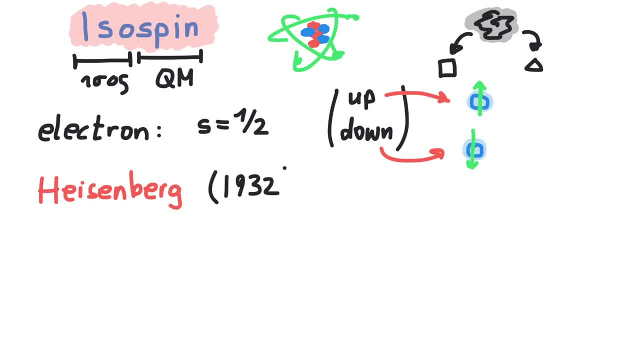 was introduced by Urbana-Heisenberg in 1932. At that time, the neutron has just been discovered and was thoroughly investigated. The neutron has approximately the same mass as a proton and the strong force acts the same between protons and neutrons. This led to the idea. 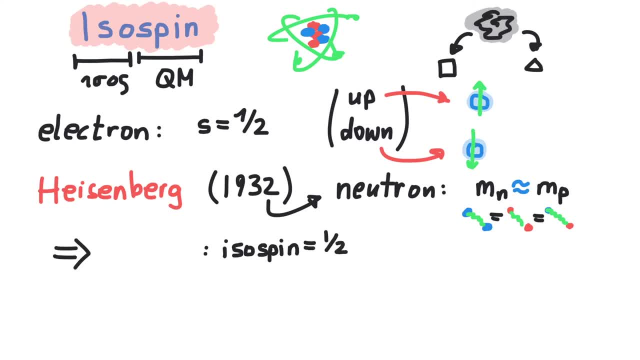 that proton and the neutron are just two realizations of the same particle, the nucleon. Just like the electron could be in an up or down state, the nucleon is just the same as a two-partylife. The nucleon has the same nel za and half- tornar to. 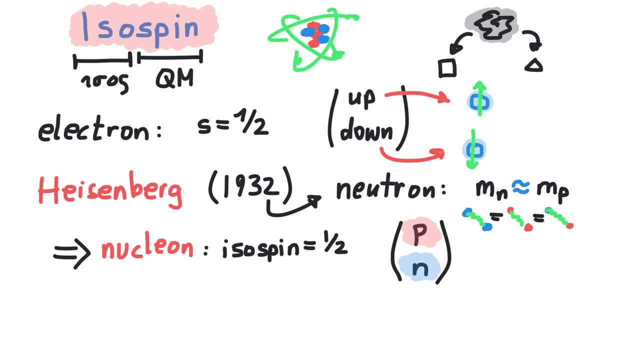 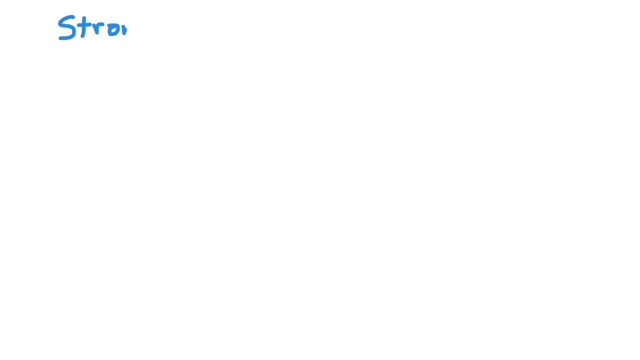 so they thought also came in a proton or neutron state. Although this idea was later replaced by the quark model, the concept of isospin continued on. Nowadays, there is strong and weak isospin. Strong isospin is assigned to the up and down quarks. 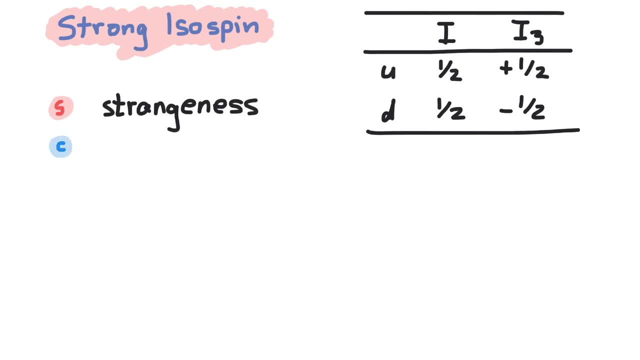 As more and more quarks were discovered and their masses were not any more comparable to the up and down mass, they have been assigned new numbers, such as strangeness, charmness, topness and bottomness. These assignment numbers are used to count the number of corresponding quarks and have 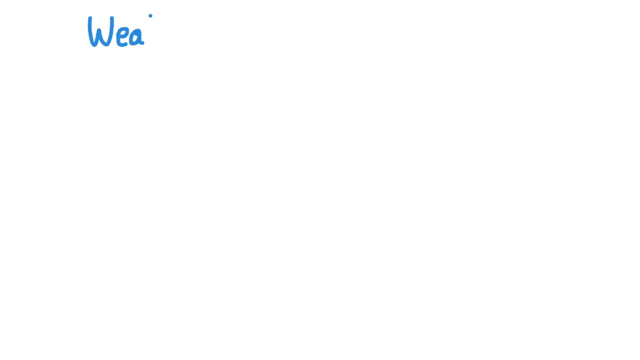 been collected in the so-called hypercharge. Weak isospin decides how a particle behaves under weak interactions, whether it can transform to another particle or if it is unaffected by weak interactions. In the context of the standard model of particle physics, the weak isospin is the charge corresponding. 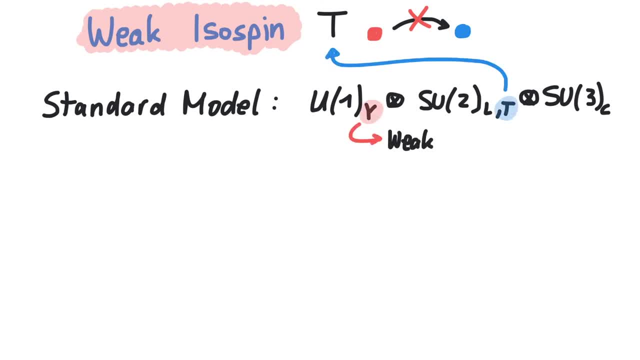 to the SU group. The so-called weak hypercharge belongs to the U. Those groups are gauge groups, That is, certain gauge groups. These gauge fields were introduced in order to ensure that the whole theory is invariant under U and SU transformations and the corresponding charges are conserved charges.